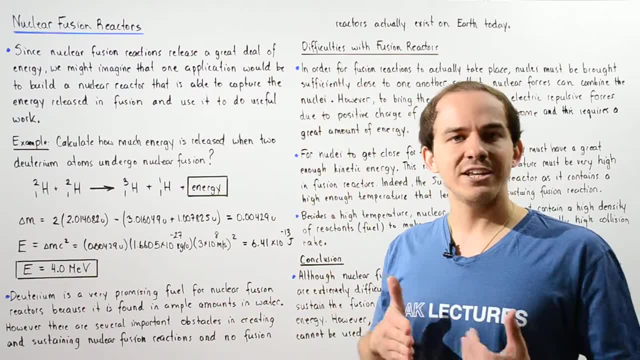 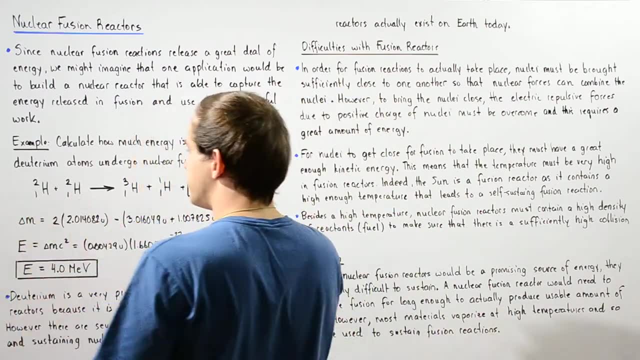 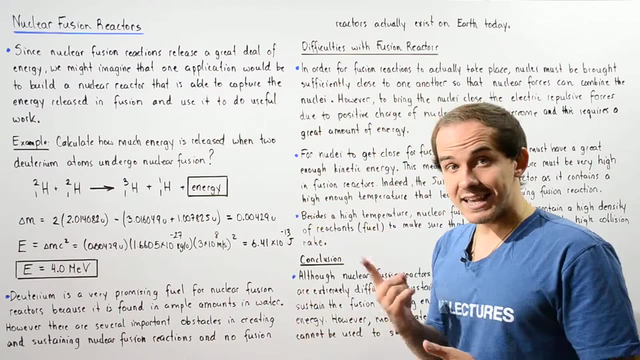 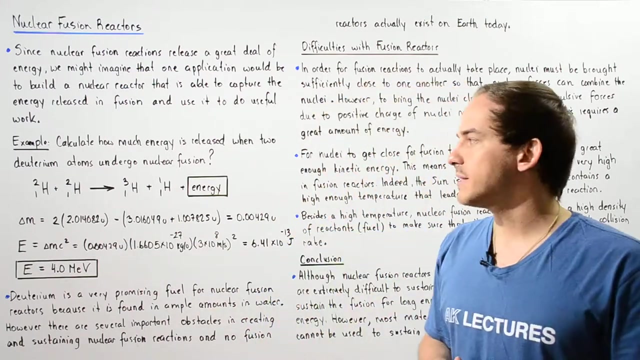 So let's begin by calculating what the change in mass is as we go from the reactant side to the product side, So as we go from these two deuterium atoms to a single tritium and hydrogen. Now recall that the mass of a single deuterium is given by 2.014082 unified atomic mass units. 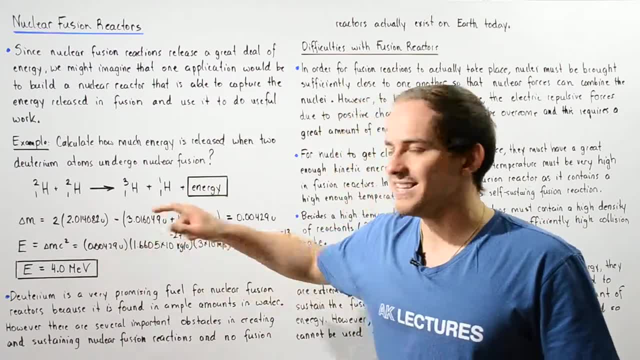 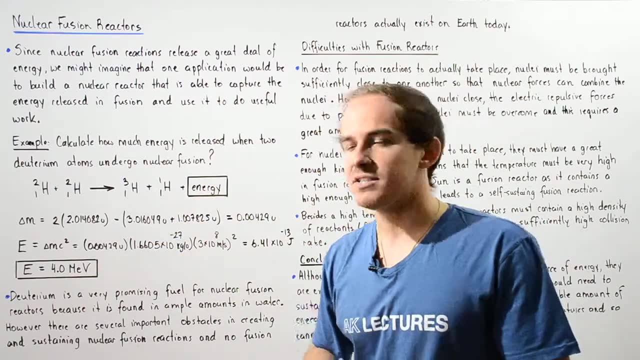 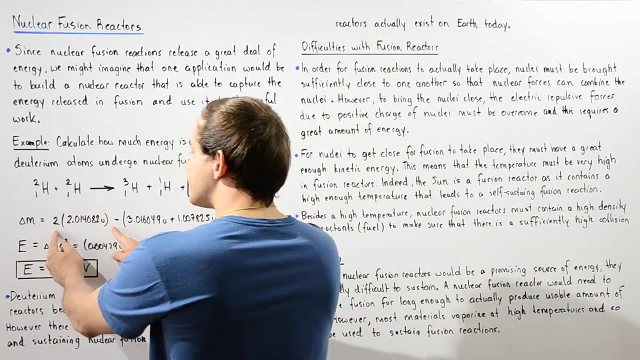 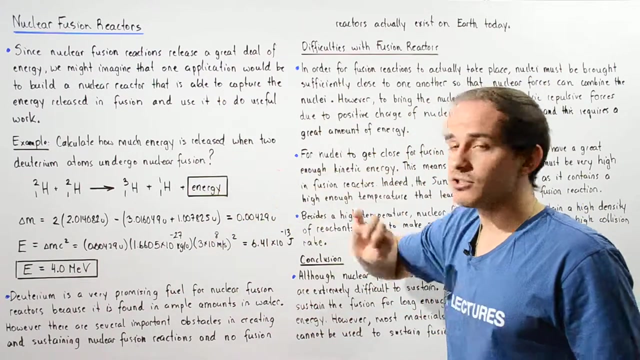 The mass of tritium is 3.016049 unified atomic mass units and the mass of our hydrogen is 1.007825 unified atomic mass units. So we take the mass of the reactants and subtract the mass of the product and we get a decrease in mass of about 0.00429 unified atomic mass units. So as we go, 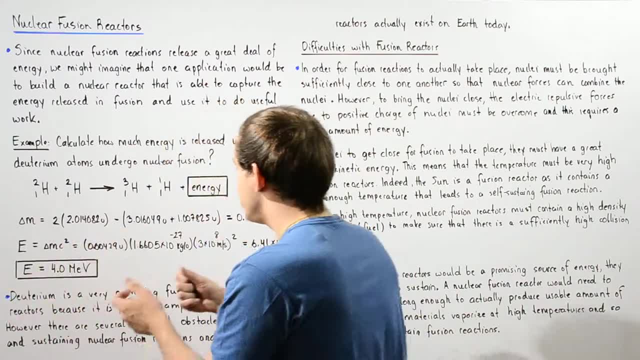 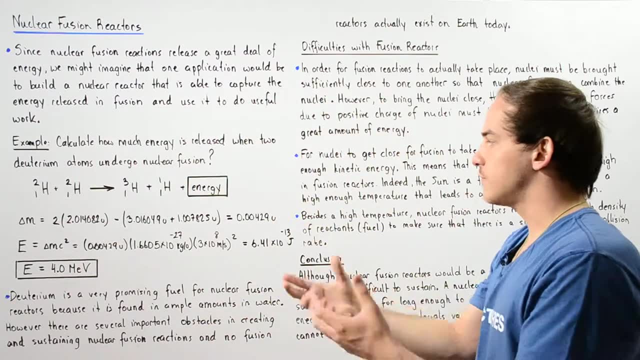 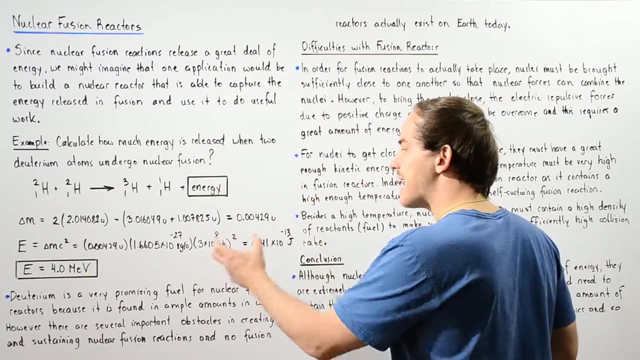 from the reactants to the products. there is a decrease in mass given by this quantity, and so energy must be released. Some of that mass is transformed into energy. Now, what quantity of energy does this decrease in mass correspond to? Well, to calculate that, we have to use the rest. 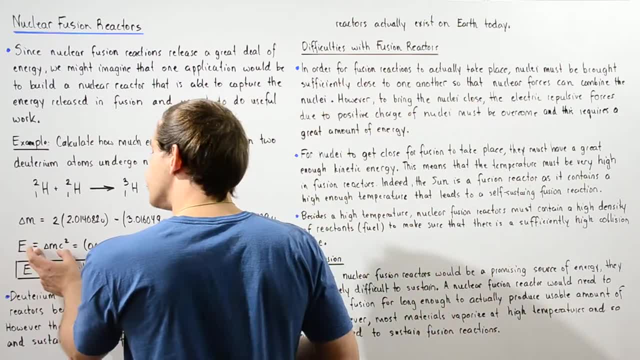 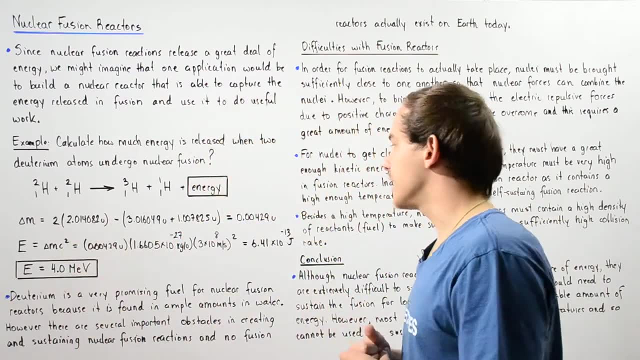 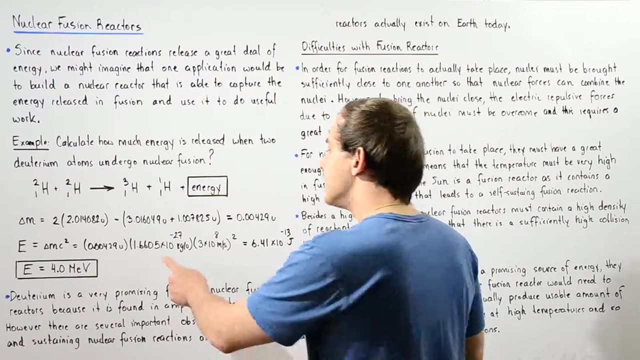 mass energy equation. So E is equal to the delta m, the change in mass in kilograms multiplied by the speed of light in a vacuum squared. So we take this, multiplied by the conversion factor of 1.6605 times 10, to the negative 27 kilograms in one unified atomic mass units and 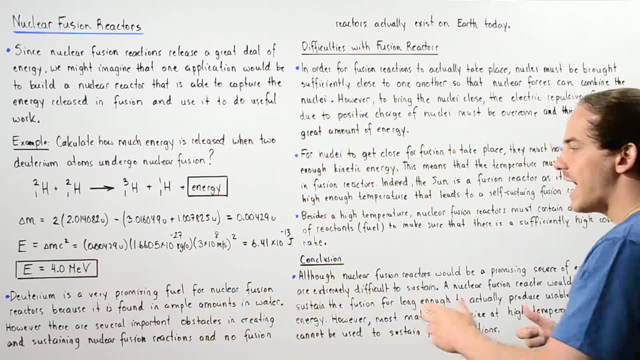 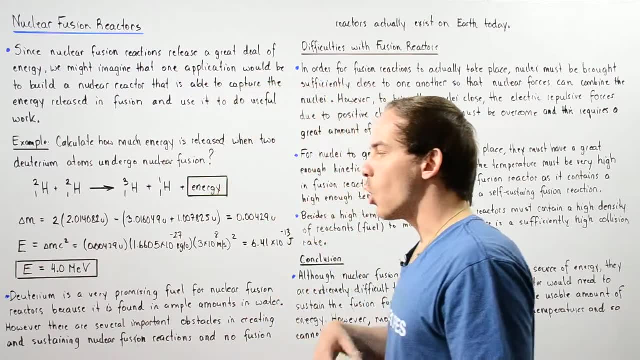 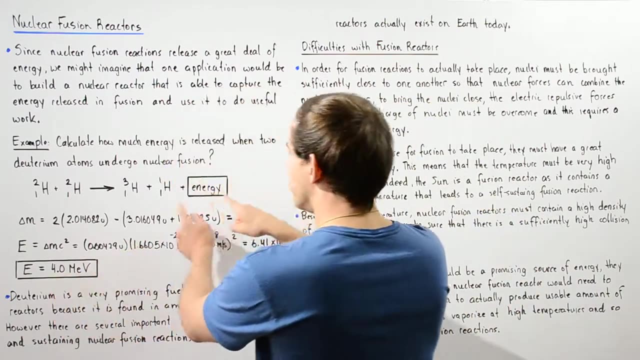 we multiply that by the squared- the speed of light in a vacuum- and we get this quantity in joules, and this is approximately equal to 4.0 mega electron volts. So this is a relatively high amount of energy that is released when we fuse these two determinants. 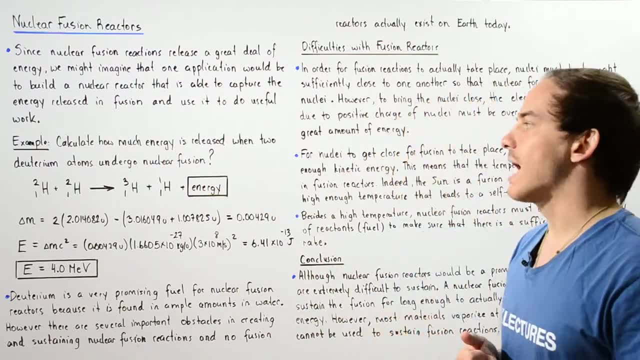 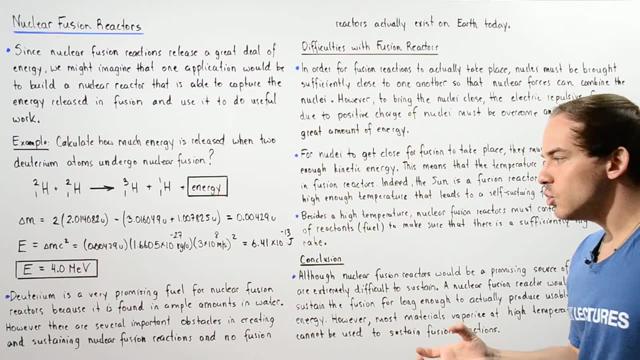 So the question is how many of these add up to the energy that we're getting? Well, the answer to this is that this is the Carnot-ulye equation, or the formula, because it's not limited to one. So if you're getting less than the current amount of energy in this, 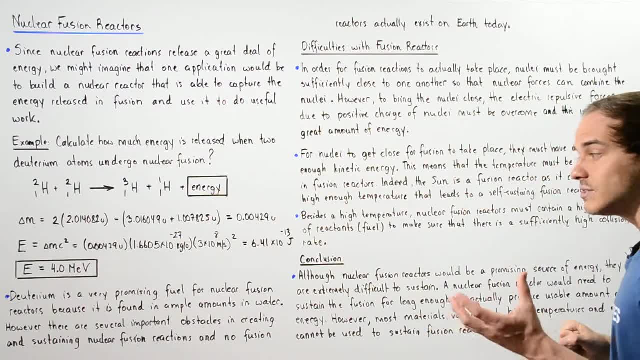 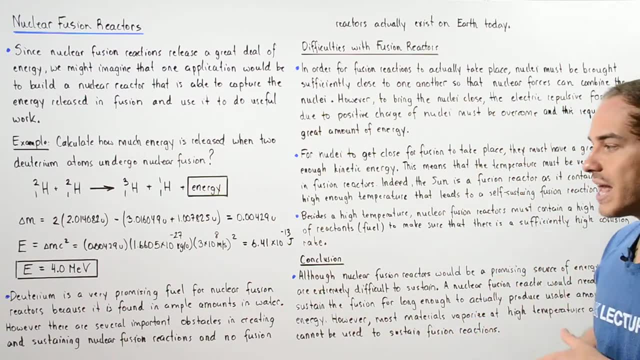 ähm address. you should remember that if you're getting less than the current amount of energy that you're getting, you should also remember that the energy in this equation is the C-radial value. if you pay a lot of attention to this equation and you get a result in this equation, 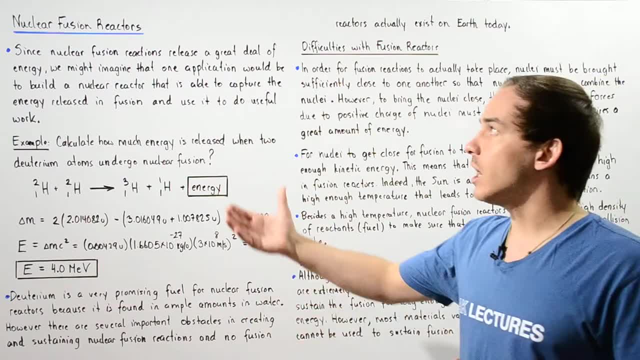 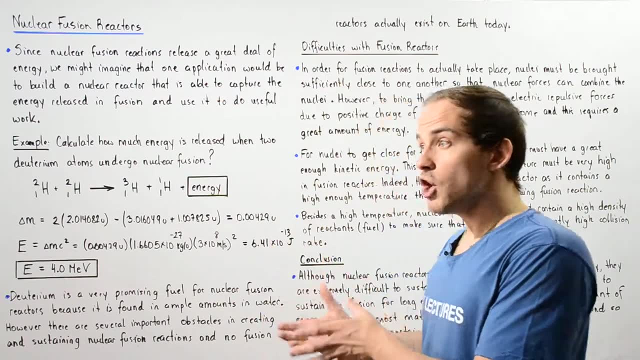 you should actually be getting that OK. so, for example, if you're getting the T-ratioum value of C-radium and you're getting the in actually producing a nuclear fusion reactor. In fact, because of these difficulties, no known fusion reactor actually exists on Earth. 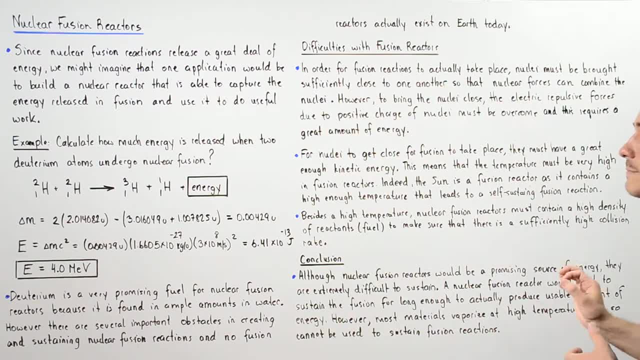 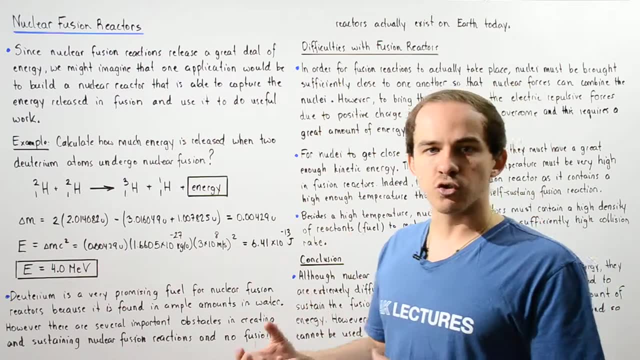 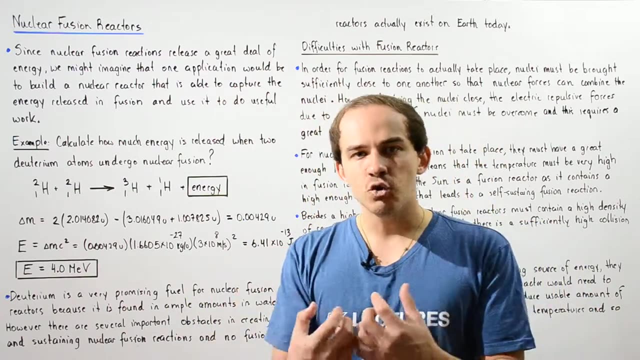 So let's actually examine these two types of difficulties. So the first difficulty is basically overcoming the electric repulsive forces that exist when we try to bring our nuclei together, to fuse them. In other words, these two deuterium atoms contain protons in the nucleus. 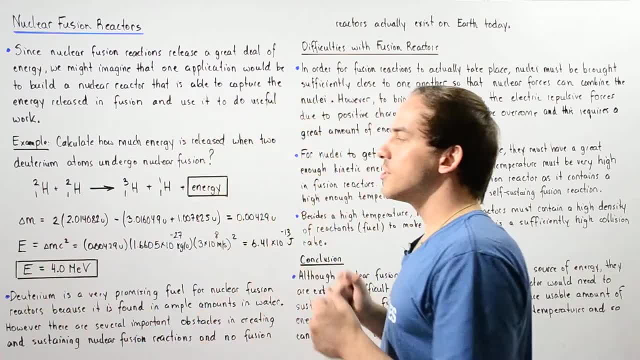 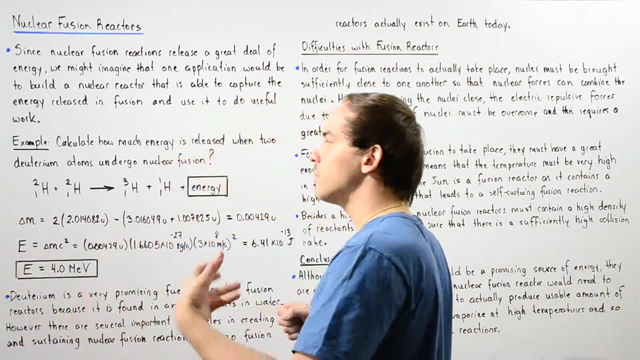 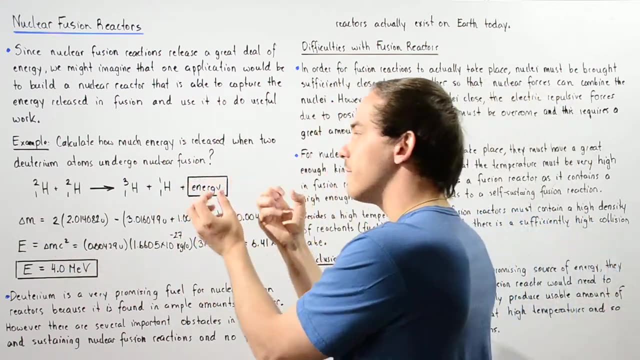 And when we try to bring these nuclei together, those two protons will basically repel one another, And as we bring them closer the electric repulsive forces increases. So that means to actually bring our two nuclei close enough for the nuclear fusion reactor to fuse them. 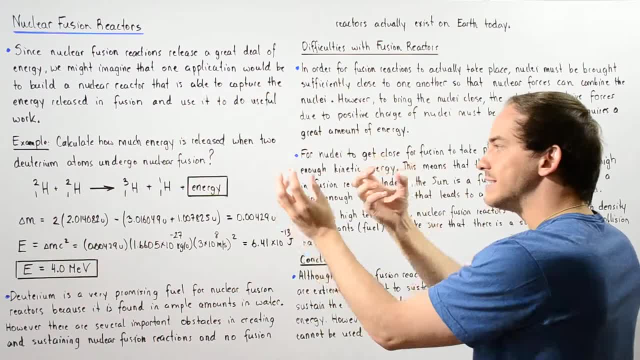 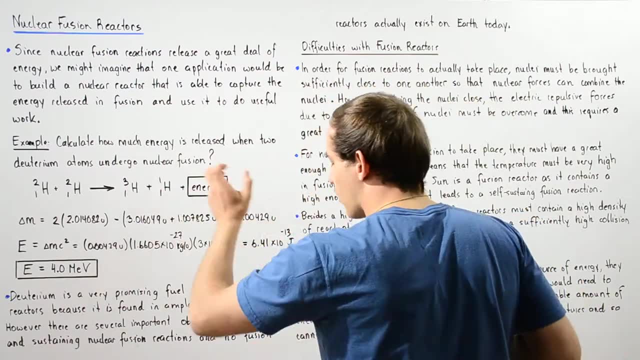 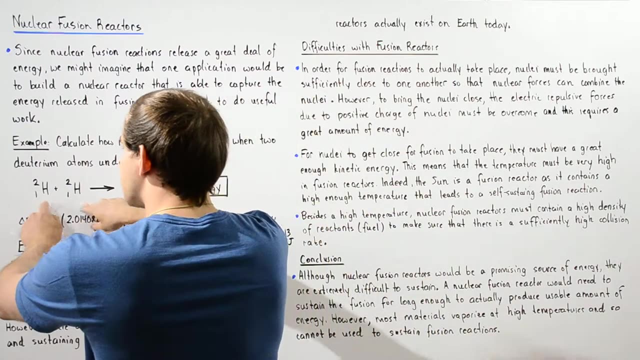 For the strong nuclear forces to actually take into place and bring and combine those two nuclei to form our tritium, releasing our hydrogen, we have to have a high enough energy. So these two H, these two deuterium atoms must have a high enough kinetic energy. 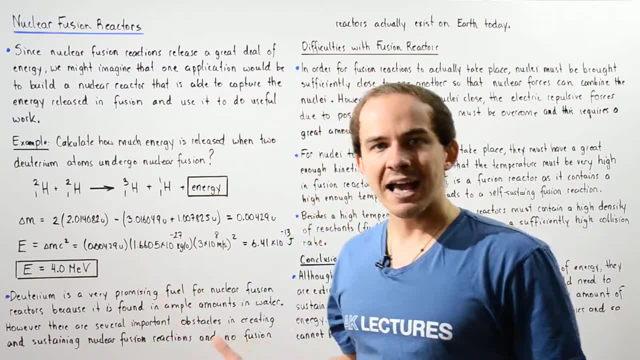 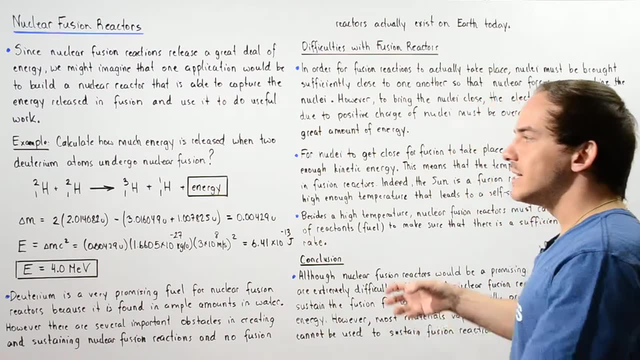 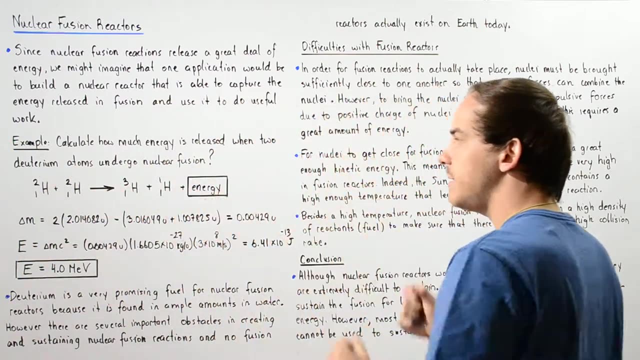 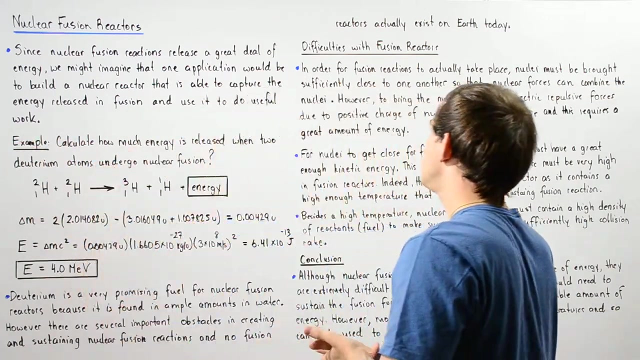 That means for the kinetic energy to be high enough, we have to have a high enough temperature. So a high enough temperature is required to actually create that fusion reaction, to actually bring our two atoms close enough, overcoming the electric repulsive forces and our strong nuclear forces, basically combine those two atoms. 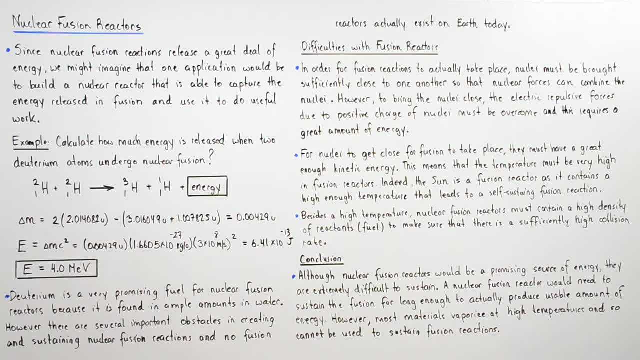 So in order for fusion reactions to actually take place, nuclei must be brought sufficiently close to one another so that the strong and weak nuclear forces can combine our nuclei. However, to bring the nuclei close, the electric repulsive forces due to the protons in the nuclei, the positive charge of those protons- 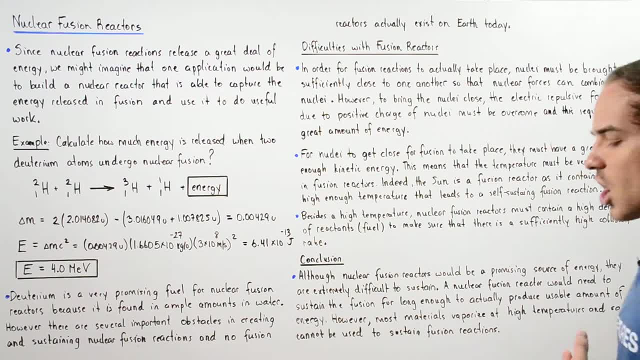 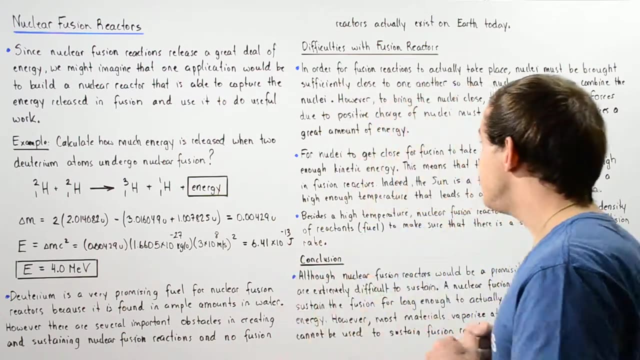 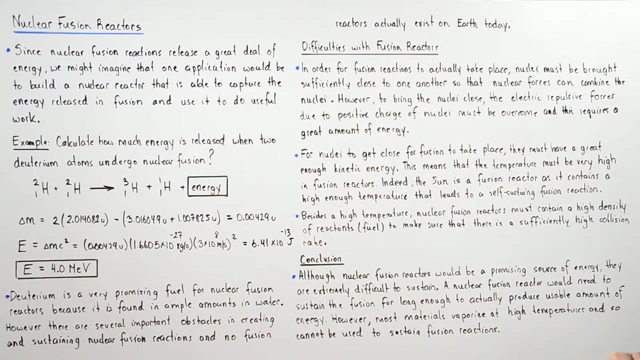 must be overcome, and this requires a great amount of energy in itself. Now, for nuclei to get close enough for fusion to take place, they must have a great enough kinetic energy. And that means because kinetic energy is proportional to the temperature, the temperature inside the nuclear fusion reactor must be high enough. 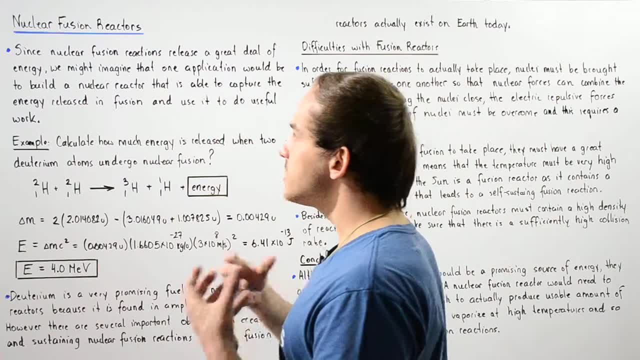 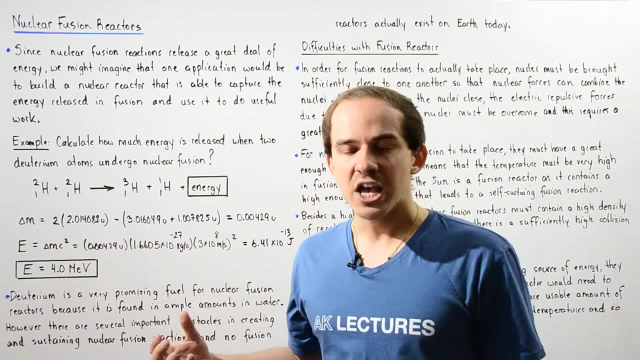 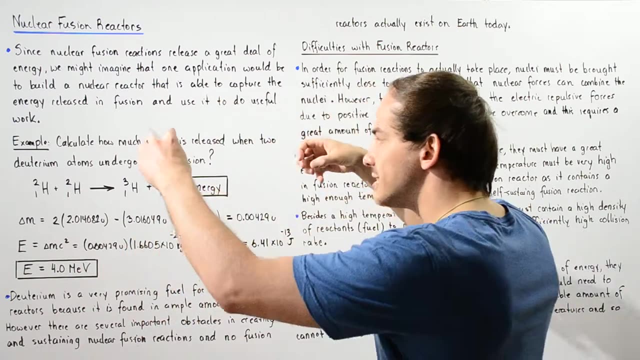 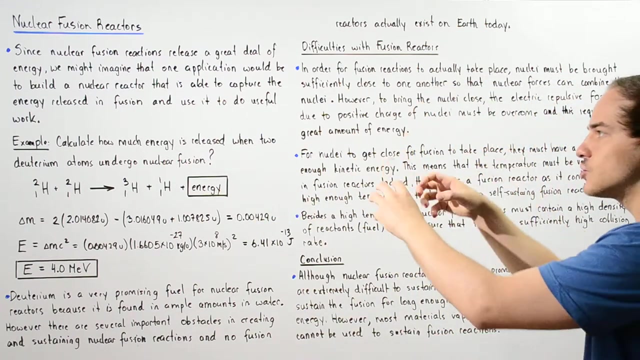 Indeed, if we examine the sun, the sun is essentially a nuclear fusion reactor in itself, And that's because it has a high enough temperature, and that high enough temperature allows our atoms to actually get close enough for fusion to take place, fusion to take place and for the strong nuclear forces to actually combine those nuclei fusing. 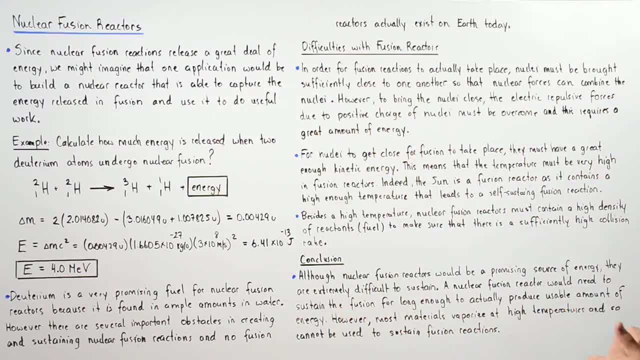 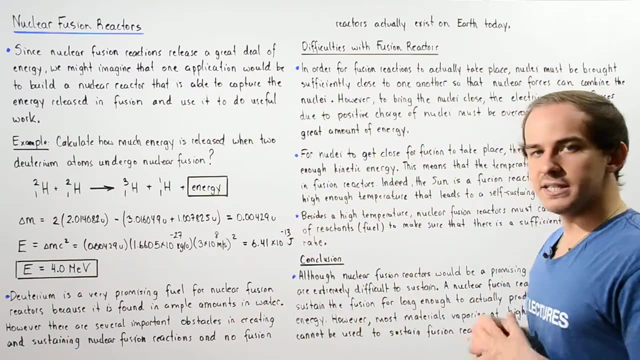 our nuclei and releasing a great amount of energy. So indeed, the sun is a fusion reactor, as it contains a high enough temperature that leads to self-sustaining fusion reaction. Now what other difficulty exists in actually creating a nuclear fusion reactor on earth? So the second type of 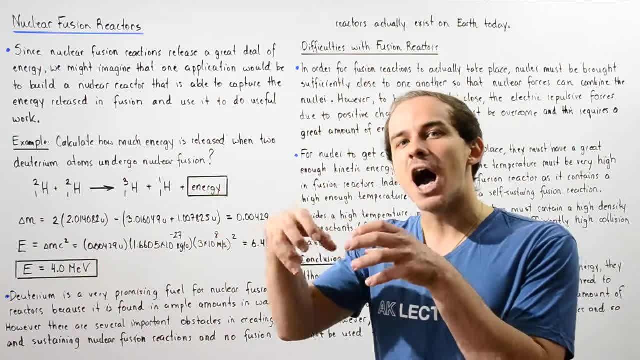 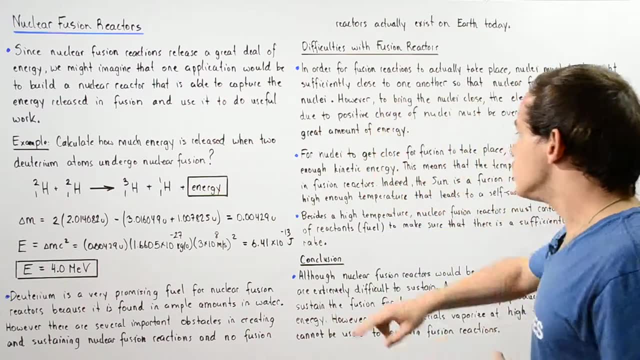 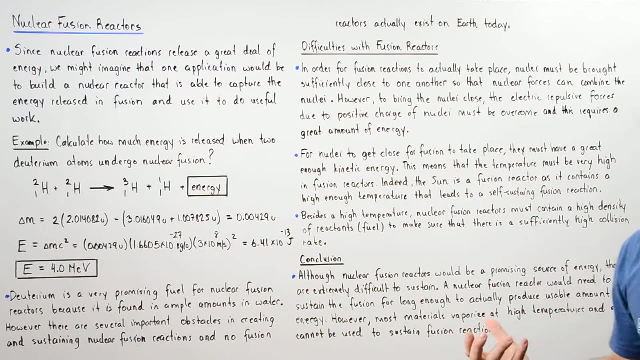 difficulty is basically placing enough of these nuclei into the reactor for our collision rate to be high enough. So, besides a high temperature, nuclear fusion reactors must contain a high density of reactants, a high density of fuel. For example, in this case, the construction of a nuclear fusion reactor is going to be a high density of fuel. So 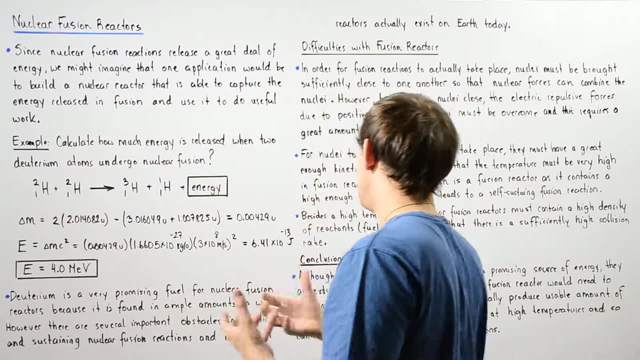 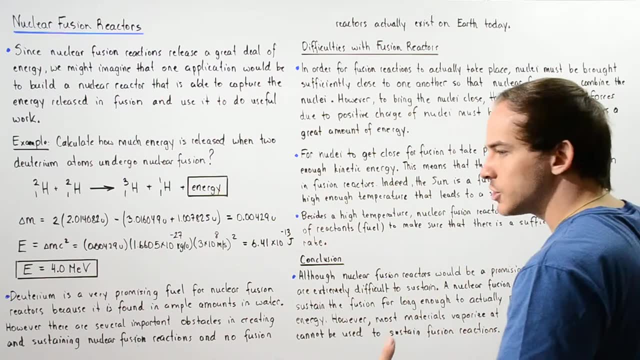 in this case the construction of a nuclear fusion reactor, is going to be a high density of fuel, So Concentration of deuterium inside the reactor must be high enough to make sure that there is sufficiently high collision rate and a sufficiently high production of energy. 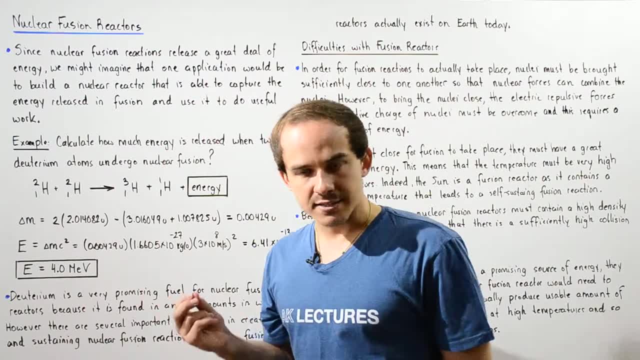 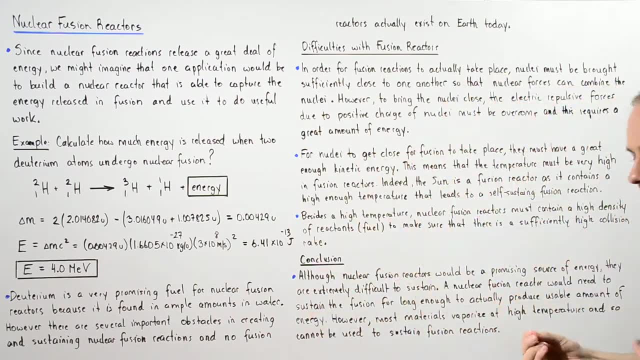 So, basically, two difficulties exist: We have the high temperature that must be obtained Inside the nuclear fusion reactor, and there must be a very high Density of our fuel. now, what exactly can we conclude about what we just discussed? so, although nuclear fusion reactors would be a very promising source of usable energy, our